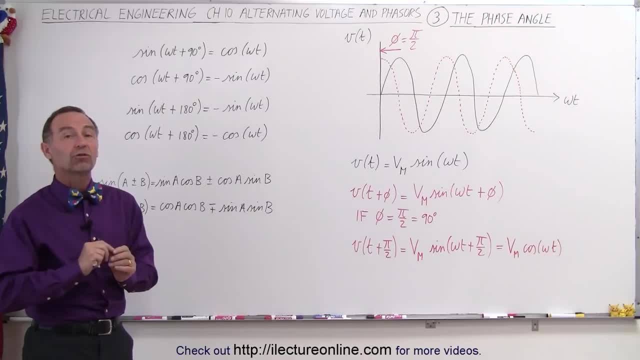 the capacitors and inductors will not be in phase with the voltage drop across the resistor. The voltage drops will either be ahead or behind in phase, and so we need to get used to using phases when we start- try to start analyzing circuits that have resistors, capacitors and inductors in. 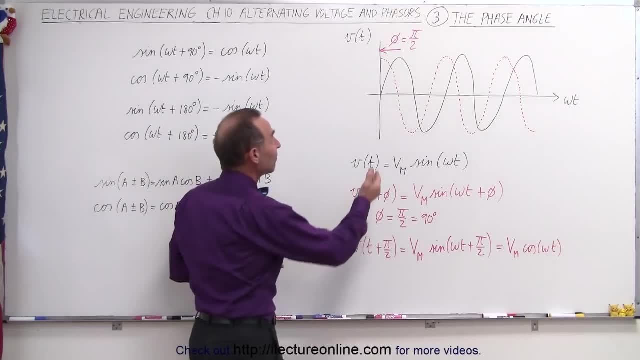 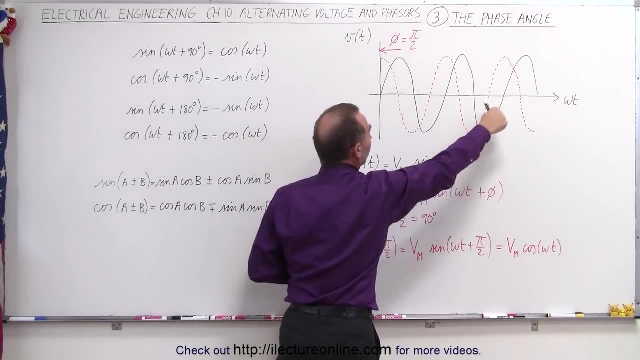 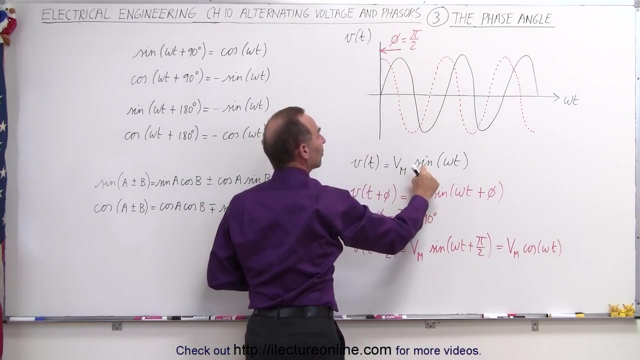 them. So here the simple concept is: let's say that the phase angle is pi over 2, which is equal to 90 degrees, If we start with the sinusoidal voltage source. and let's say in this case, this is the voltage as a function of time- this is the black curve- is equal to the maximum voltage times the. 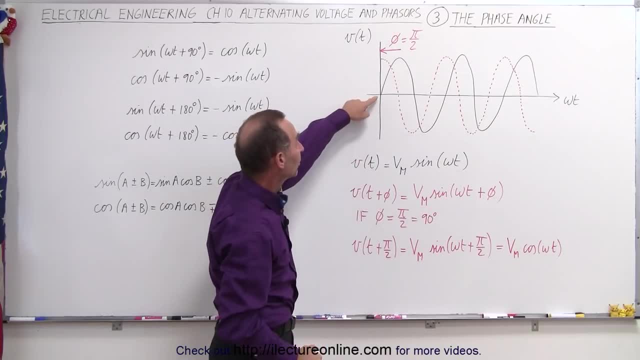 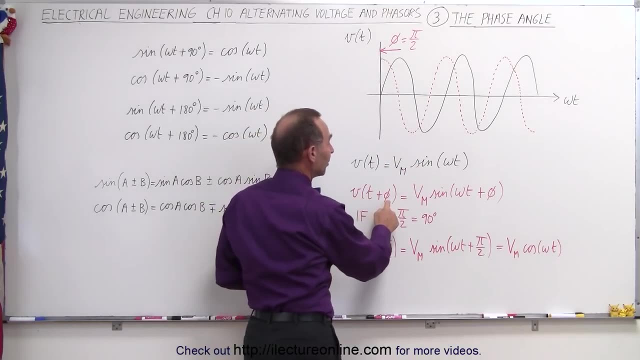 sine of omega t. We use the sine here because when t is equal to zero, the value is zero and of course, c of zero is equal to zero. So this is the sine of omega t and this is the sine of omega t. So is zero. so that matches. but what if we now add a phase angle? well, that will shift the curve to the. 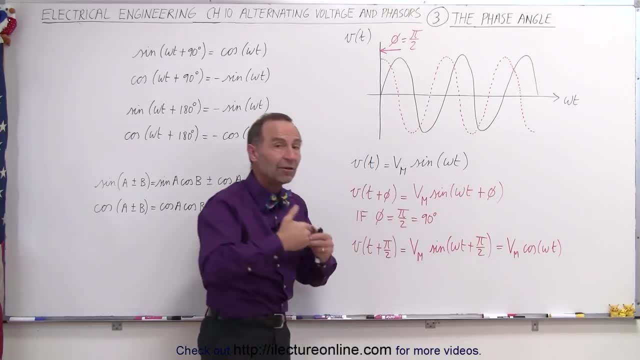 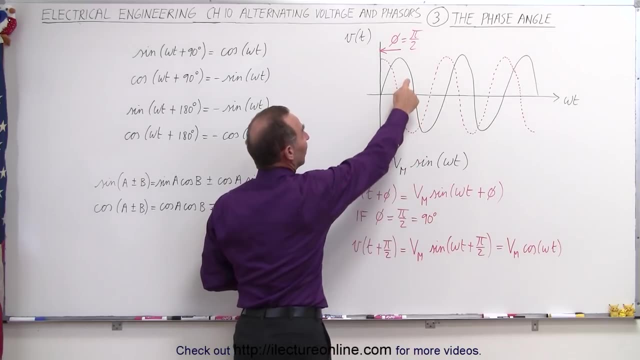 left. if we add a positive phase angle, that means we get to the maximum voltage a little bit more quickly, and if the phase angle equals pi over 2, which is 90 degrees, the sine function simply becomes a cosine function, which means that if we have a voltage source that has a phase angle of 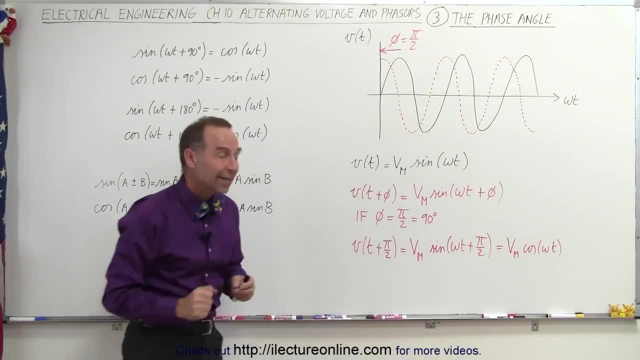 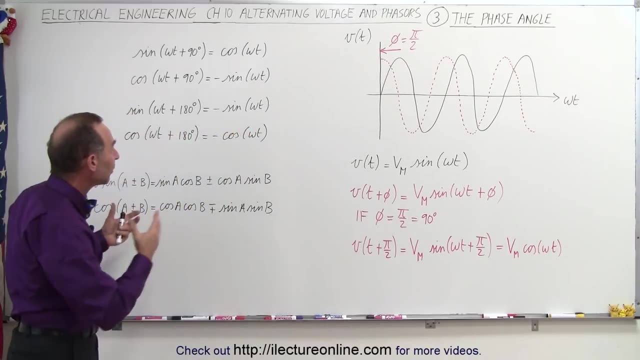 90 degrees. so we add pi over 2 to omega t, then the sine function simply becomes a cosine function of omega t. so it helps us to be able to go back and forth between sine and cosine functions by looking at the phase shifts. so here we can see that if we add 90 degrees to the sine function, 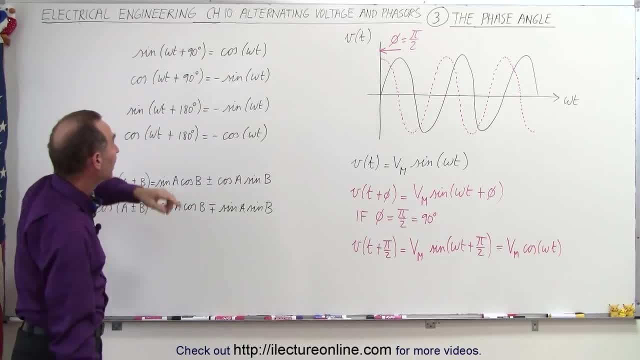 we get the positive cosine function. however, if we add a 90 degree phase angle to the cosine function, we get the negative sine function. with other words, it kind of flips over the sine function and you can see that if we take the red curve here and move it to the left, another pi over 2. 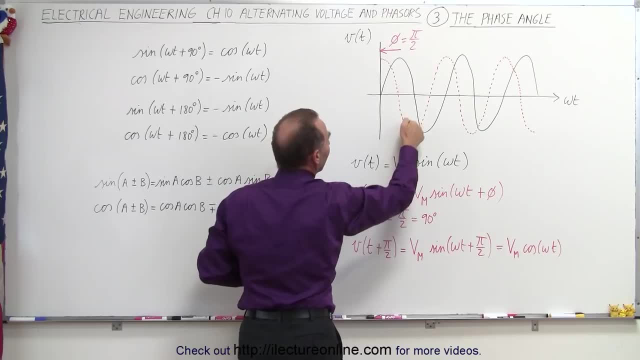 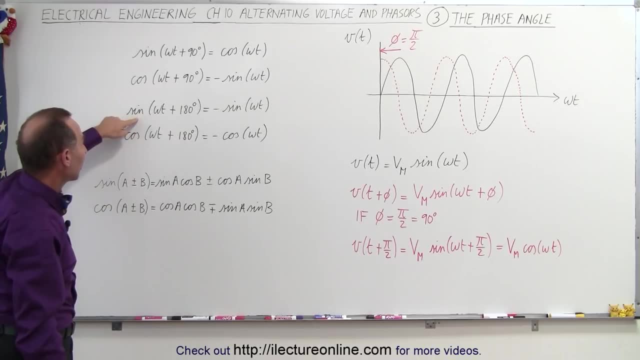 then you can see that by the time we get over here we're on the way down and we have a complete opposite function as the sine function, therefore the negative sine function. Also notice that if we have a sine function, we had 180 degrees pi. that gives us the negative. 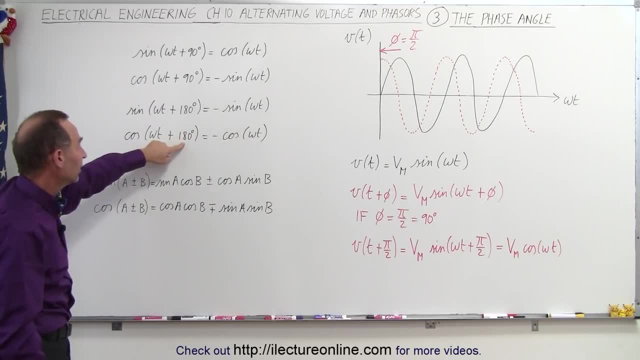 sine function and if, with a cosine function with a phase angle of 180 degrees that gives us the negative cosine function, it simply flips the function over graphically. It also might help if we remember the identities that the sine of a plus b and the cosine of a plus b can. 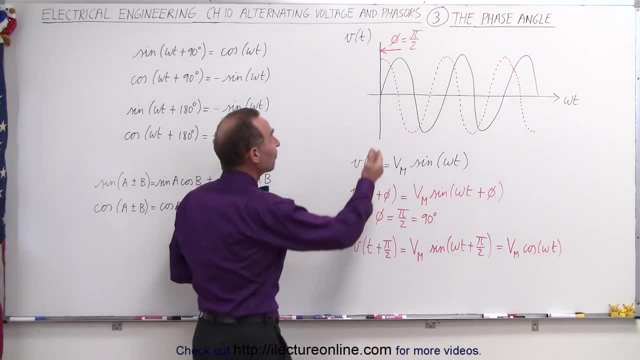 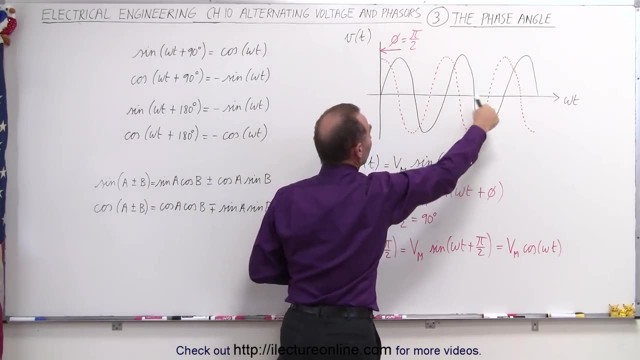 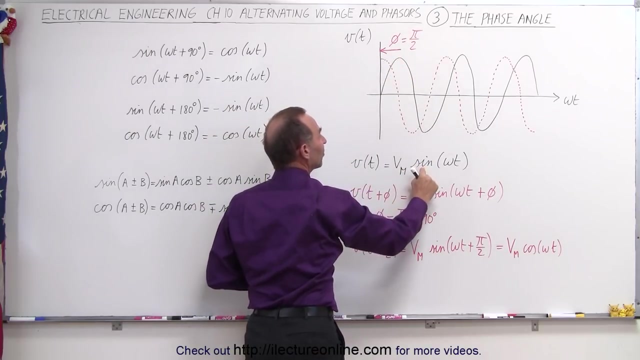 them. So here the simple concept is: let's say that the phase angle is pi over 2, which is equal to 90 degrees, If we start with the sinusoidal voltage source. and let's say in this case, this is the voltage as a function of time- this is the black curve- is equal to the maximum voltage times the. 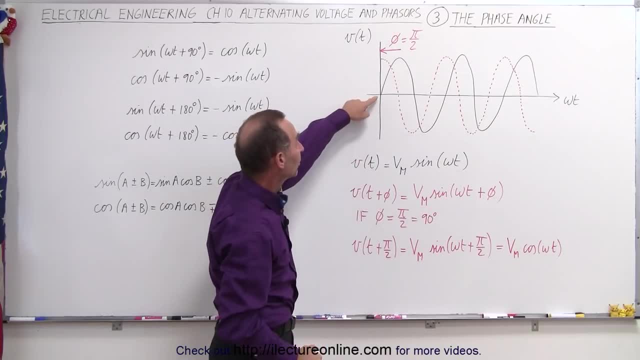 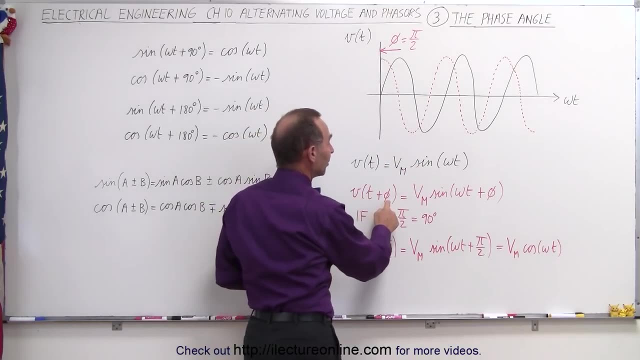 sine of omega t. We use the sine here because when t is equal to zero, the value is zero and of course, c of zero is equal to zero. So this is the sine of omega t and this is the sine of omega t. So is zero. so that matches. but what if we now add a phase angle? well, that will shift the curve to the. 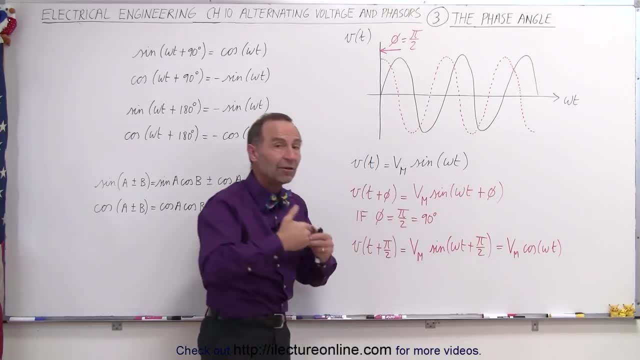 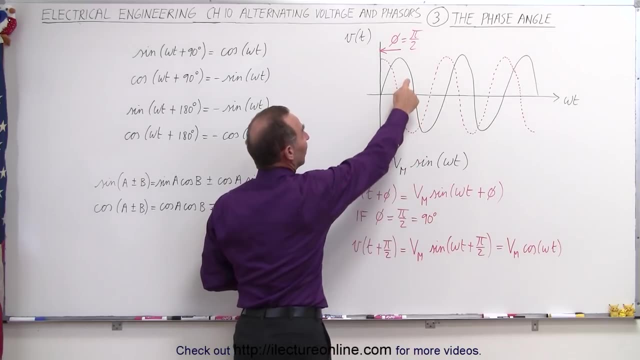 left. if we add a positive phase angle, that means we get to the maximum voltage a little bit more quickly, and if the phase angle equals pi over 2, which is 90 degrees, the sine function simply becomes a cosine function, which means that if we have a voltage source that has a phase angle of 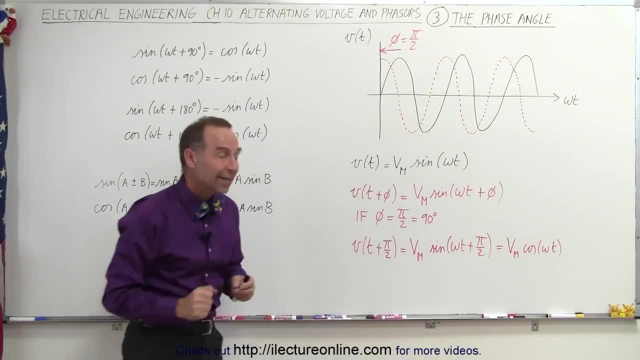 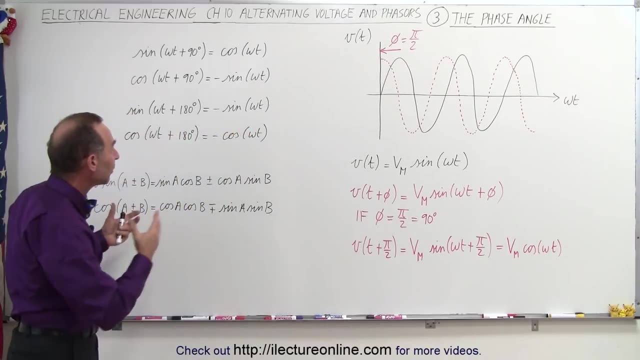 90 degrees. so we add pi over 2 to omega t, then the sine function simply becomes a cosine function of omega t. so it helps us to be able to go back and forth between sine and cosine functions by looking at the phase shifts. so here we can see that if we add 90 degrees to the sine function, 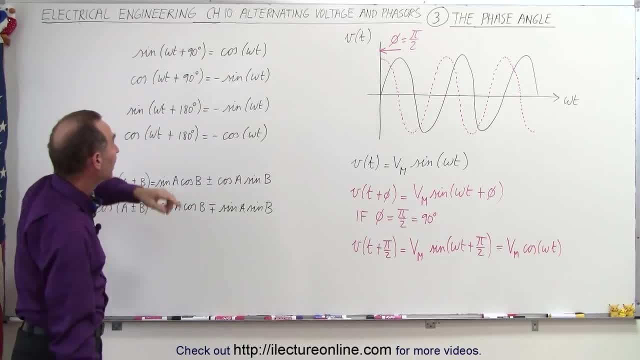 we get the positive cosine function. however, if we add a 90 degree phase angle to the cosine function, we get the negative sine function. with other words, it kind of flips over the sine function and you can see that if we take the red curve here and move it to the left, another pi over 2. 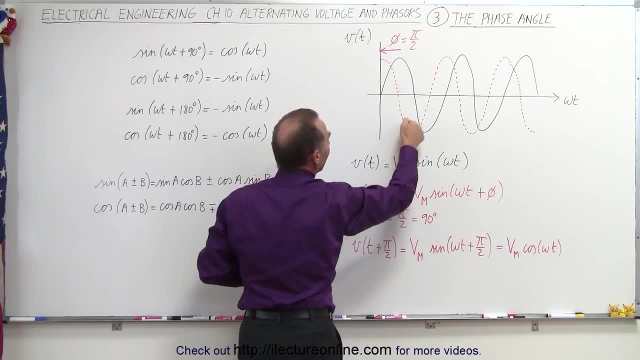 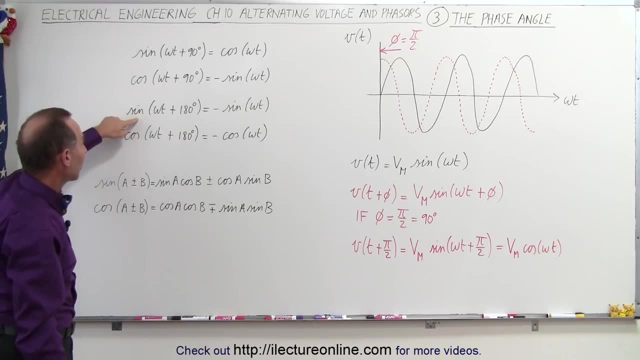 then you can see that by the time we get over here we're on the way down and we have a complete opposite function as the sine function, therefore the negative sine function. also notice that if we have a sine function, we had 180 degrees pi. that gives us the negative sine function. and if we 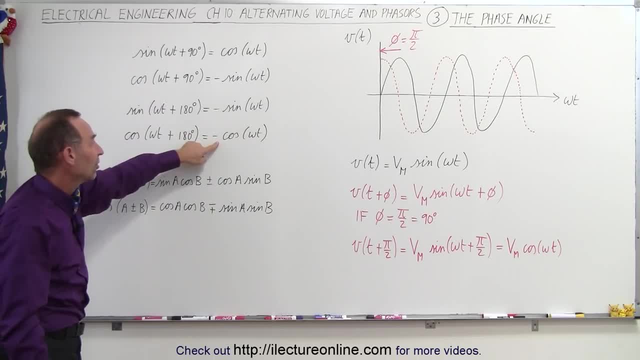 the cosine function with a phase angle of 180 degrees. that gives us the negative cosine function. it simply flips the function over graphically. it also might help if we remember the identities that the sine of a plus b and the cosine of a plus b can be the cosine of a plus b. 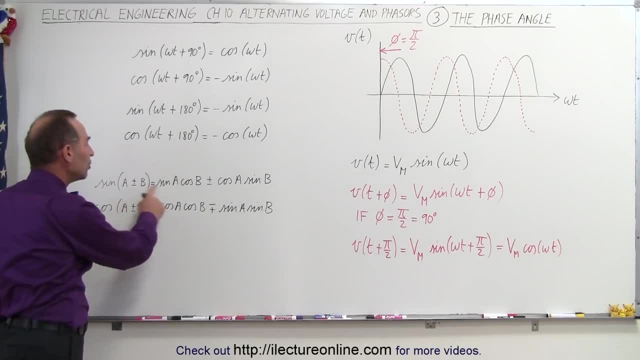 can be written as follows: notice that if it's a plus b, notice the plus here still remains a plus. so we have the sine of a times the cosine of b plus the cosine of a times the sine of b, and we have a minus here, we get a minus there. but when we add angles, when we have the cosine,